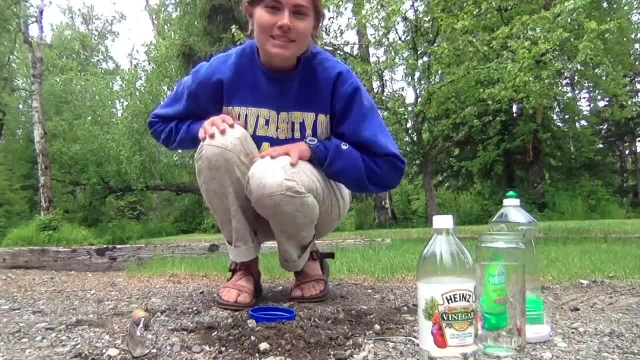 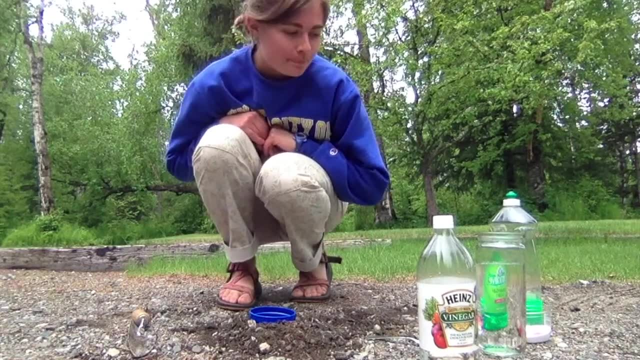 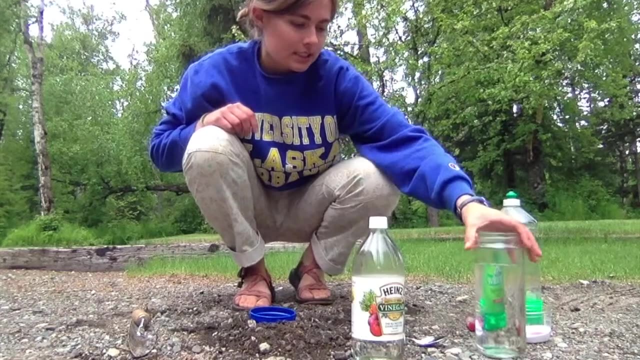 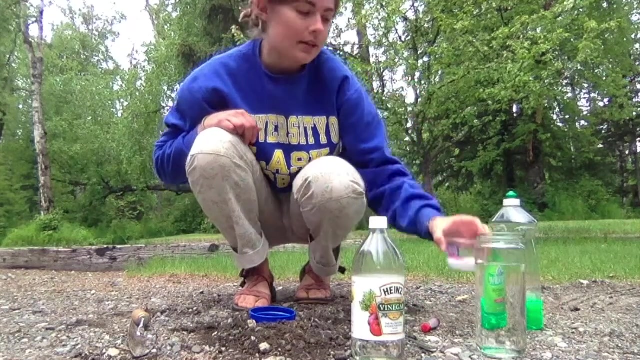 Hi, I'm Ellie. I'm a senior environmental studies biology major at Whitman, and today I'm going to show you how to build and set off a volcano. So what you're going to need is you're going to need vinegar water, a spoon to mix with food coloring, baking soda. 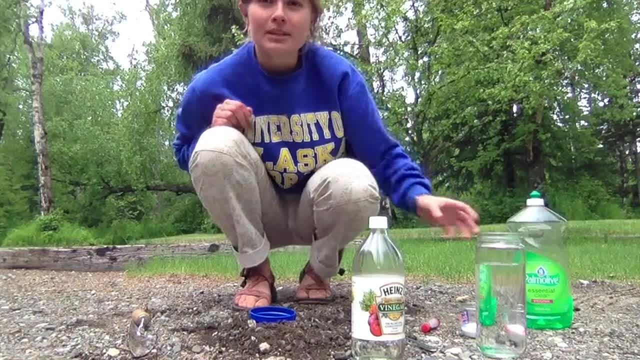 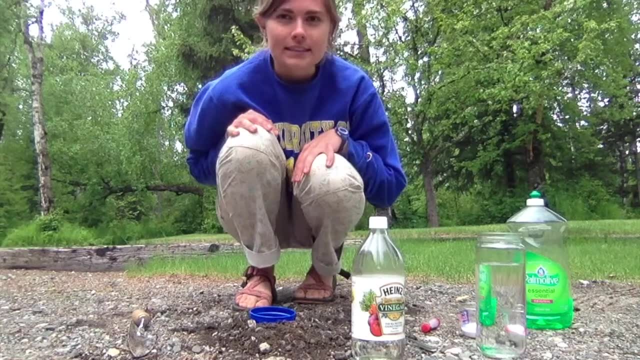 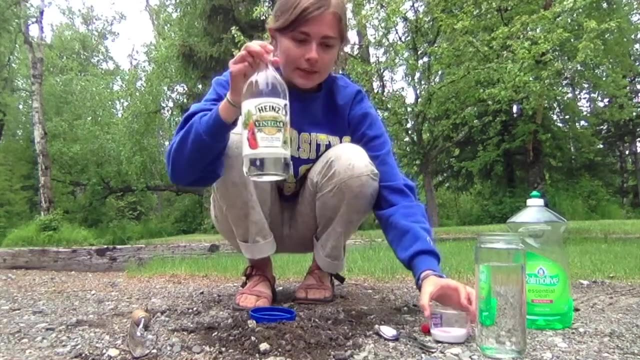 dish soap, and I recommend doing this experiment outside because it can get a bit messy. And, briefly, the science that's going on here is that it's an experiment, a reaction taking place between the baking soda and the vinegar, And so first I built up my volcano and I put a 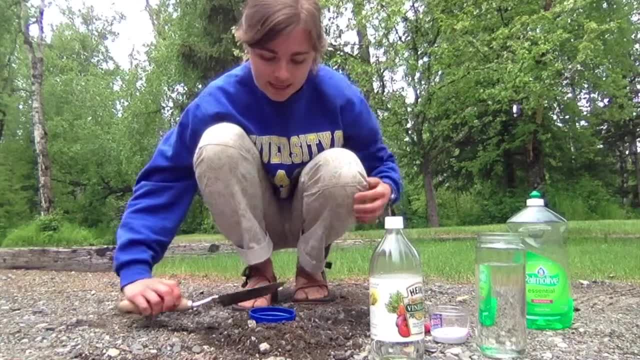 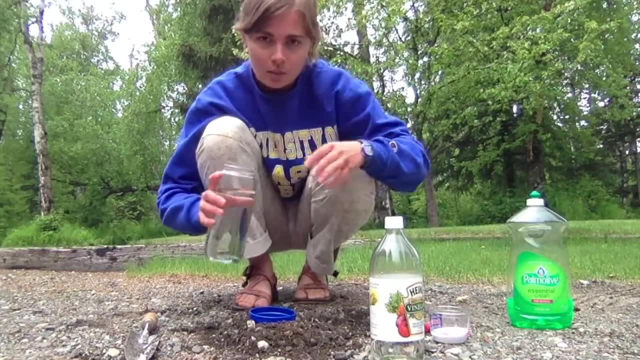 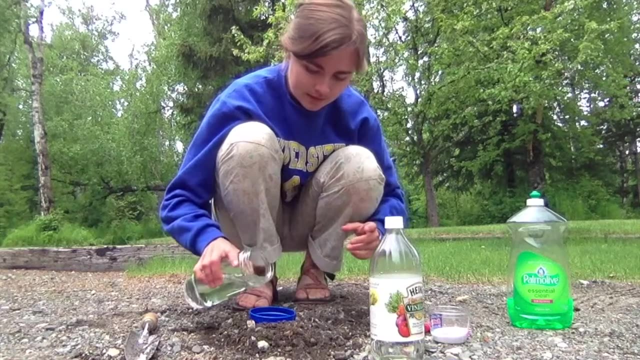 cup in here where the reaction is going to take place, and I want to make sure that the cup isn't going to tip over, And so first I'm going to add water to my cup until it's about two-thirds full, And then I'm going to add a squirt of dish soap. 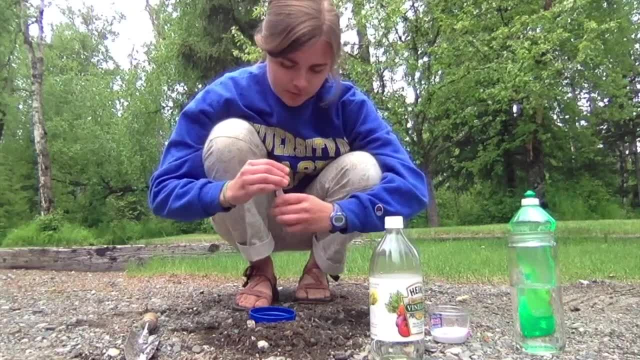 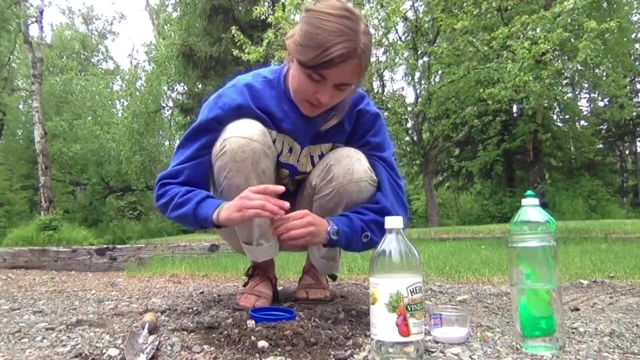 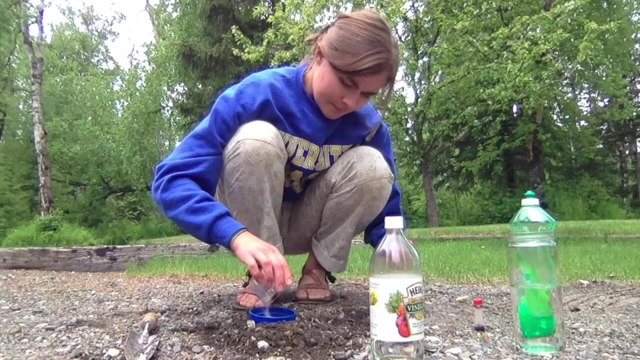 And then I'm going to add a little bit of food coloring- and I'm using red, but you can use whatever color you want- And then I'm going to add my baking soda And then I'm going to give it a nice, good stir. 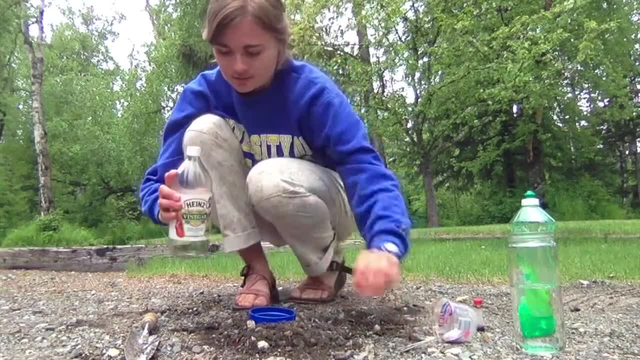 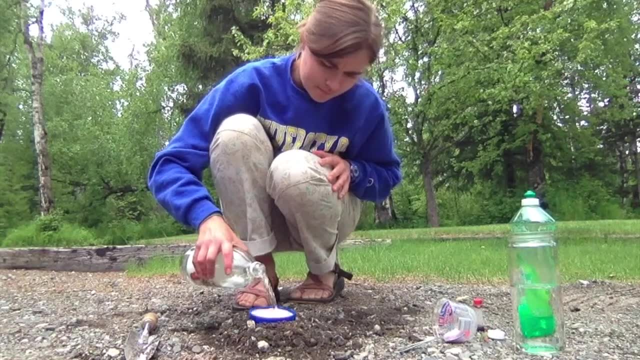 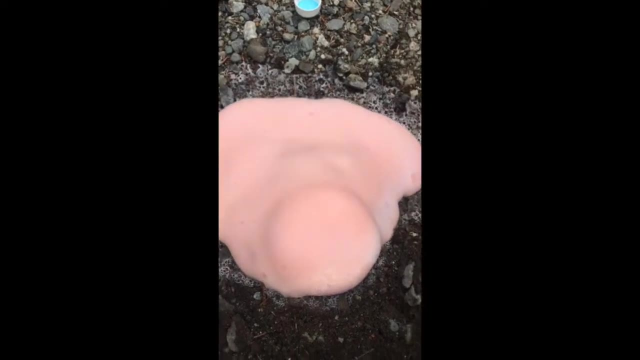 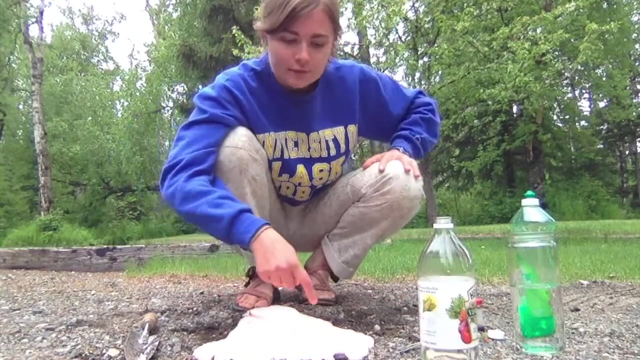 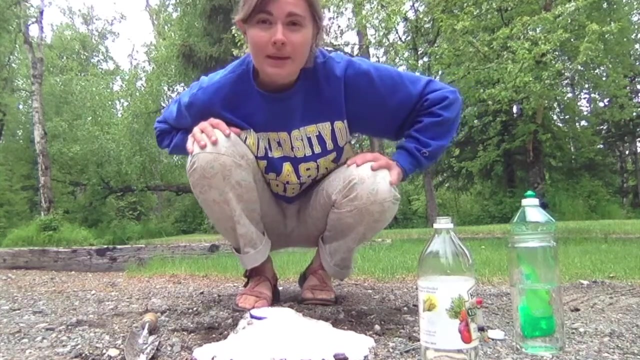 And now it's time to add the final ingredient, the vinegar, And look, it's exploding. So what's going on is all these bubbles in the foam that's coming up is the reactions taking place between the vinegar and the baking soda, because it's an interaction between a base and an acid. Thanks for watching.